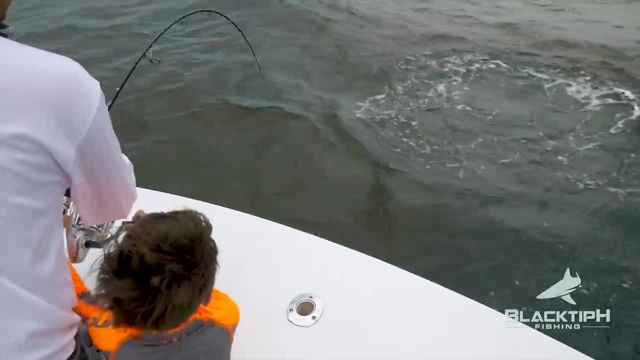 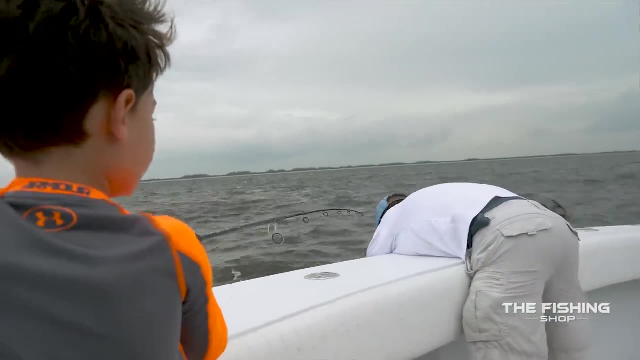 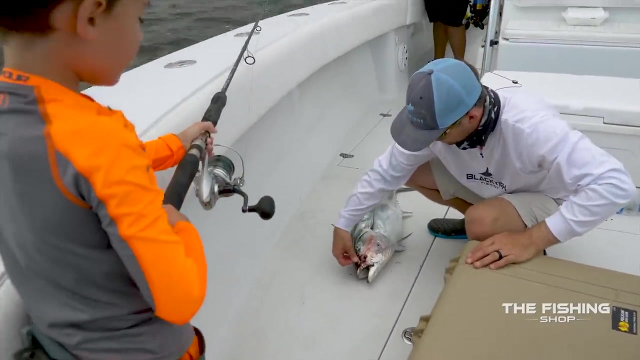 Hold on, Hold on, Ready, I need you to hold that rod. Hold that rod Right buddy. Hold the rod right there. That's a big finito. Look at that Right there. All right, man, So we successfully. 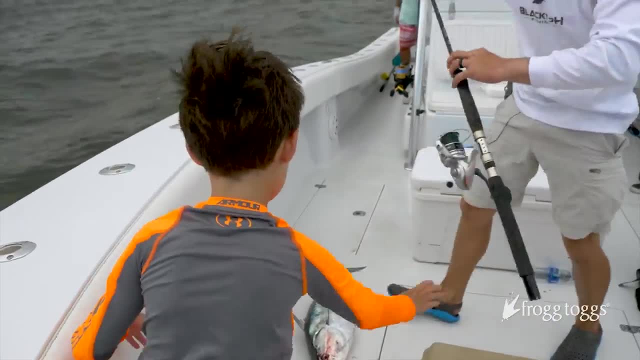 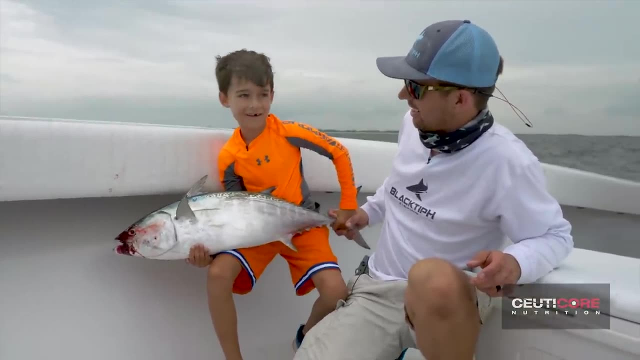 have caught the next fish in the food chain. You want to hold them up. That fish is almost as big as you are, dude. That's the bait, Isn't that crazy? What do you think is going to come and eat this thing? Shark, You think a shark? 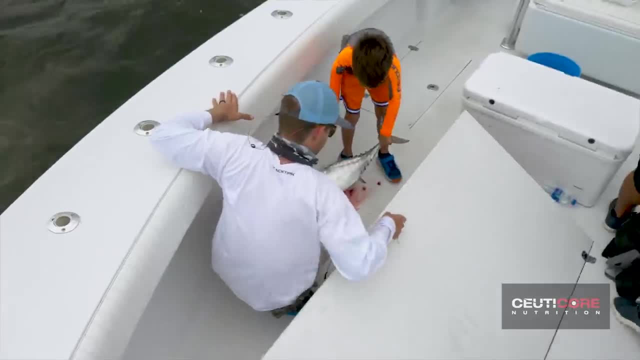 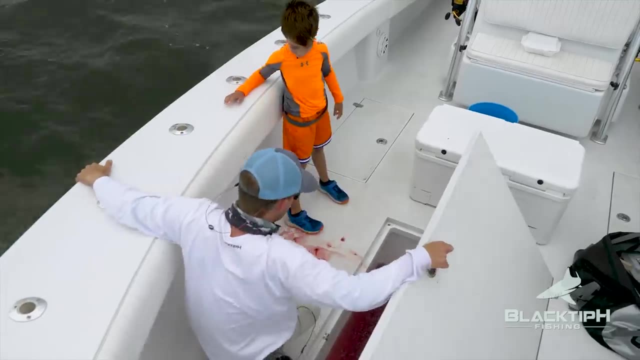 Something very big. I can tell you that Something very, very big. It's going to be very cool. Put him in there, Vy. There he goes, Sweet man. Next step in the food chain. Me and Vy are going to have a competition right now to see who can catch a bait faster. 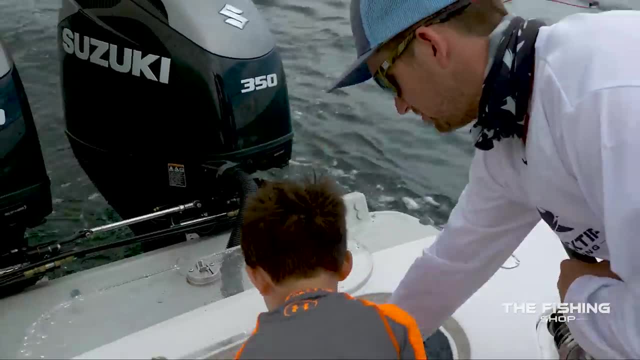 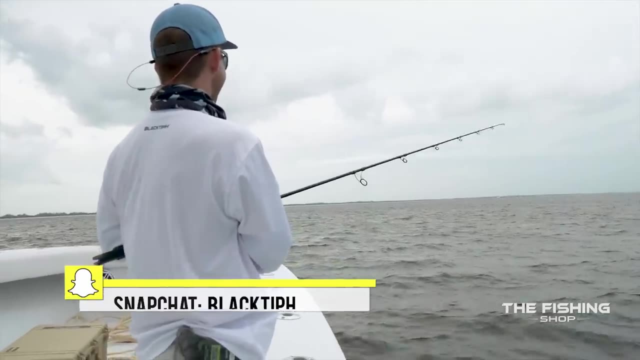 with one hand. You ready. Vy You going to win? Vy Ready. All right, let's go. Smoked, Absolutely smoked me. That's why he was screaming so hard. What the Goliath or the Bonita? 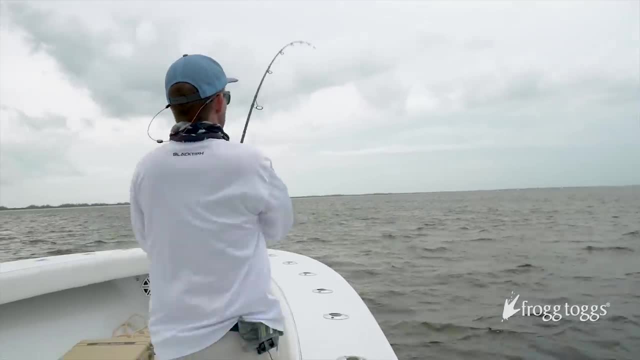 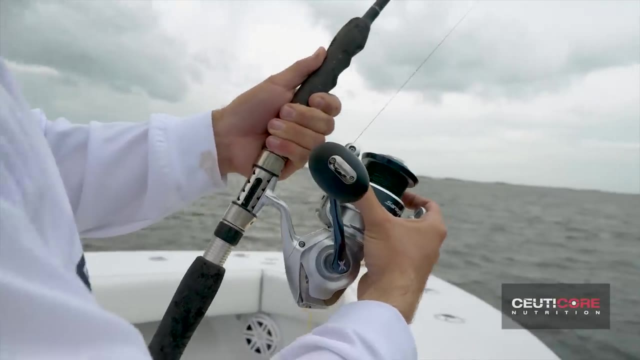 Yeah, he's like: yeah, Oh, he's got a bite, He's got a bit up There, we go Bonita on Hold on Bonita. Oh my gosh, Oh my gosh, Dude, he's smoking me. I can't stop him. 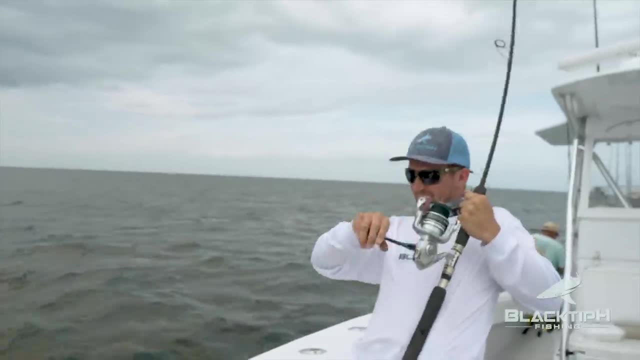 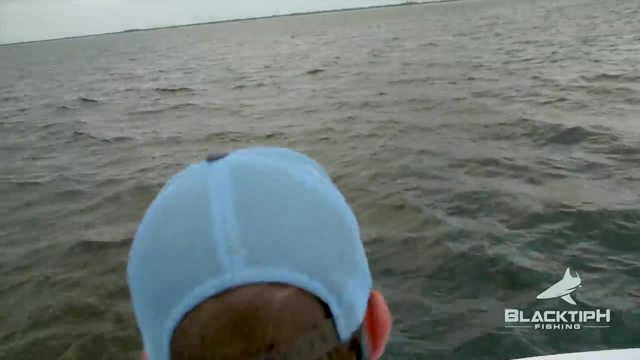 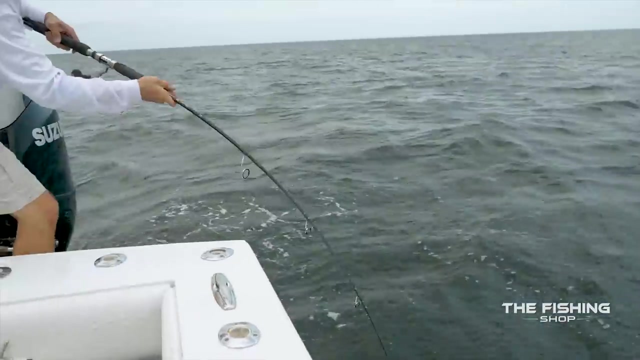 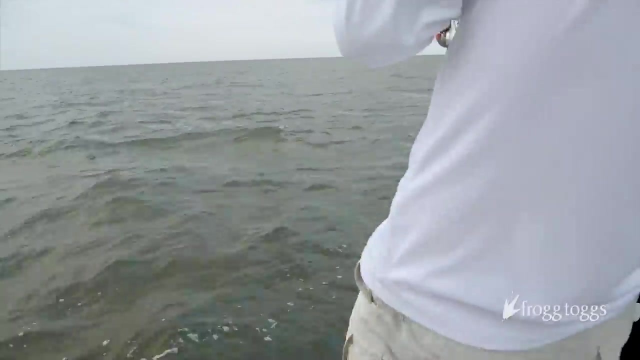 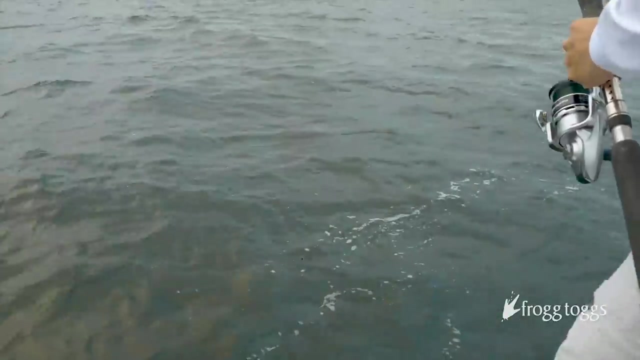 That's unbelievable. He's getting chased 100%. It's a Goliath on him. There's a Goliath on him. Dang No dude. He was just doing: Oh my gosh, Oh my gosh, dude. 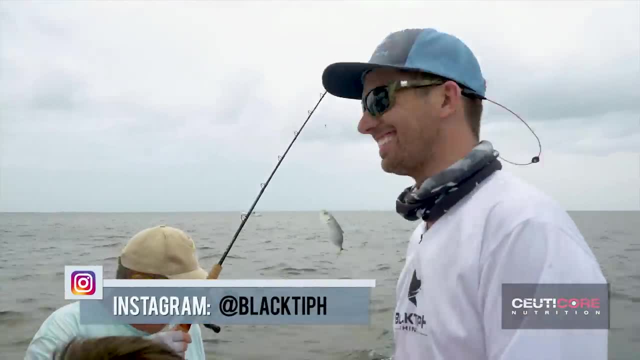 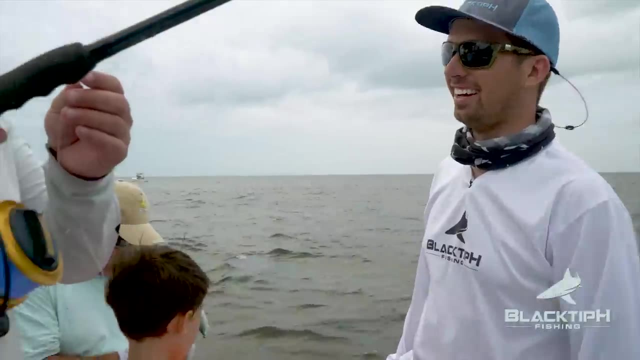 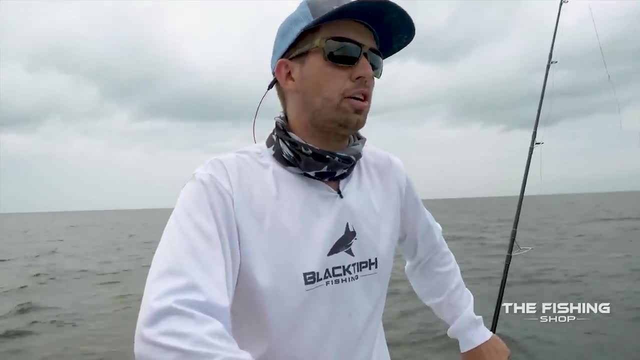 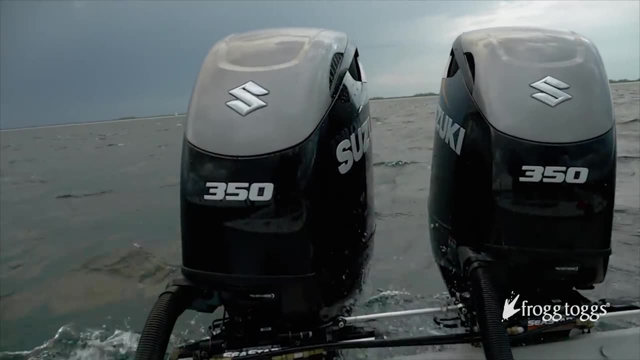 You know what's funny? A 20-pound Bonita. I don't care how experienced you are, I don't care how strong you are, I'll take the breath out of you. You think it's going to get hit? Yeah, 100%. 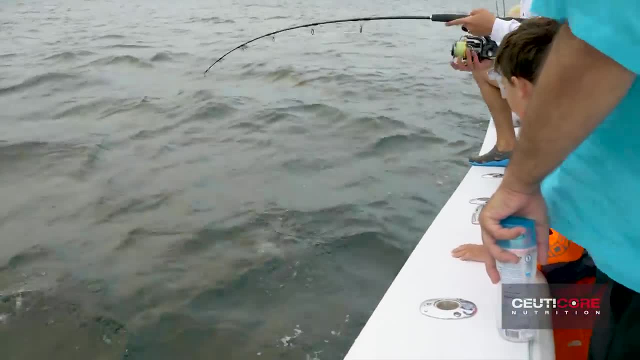 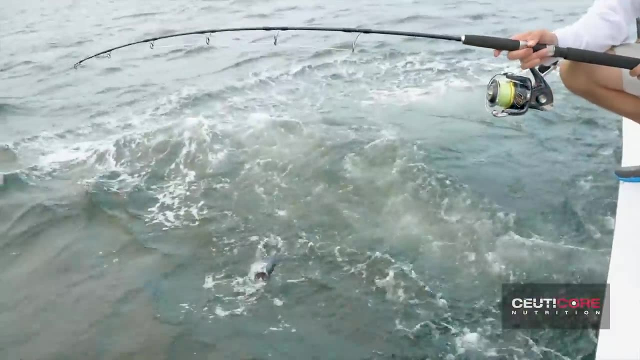 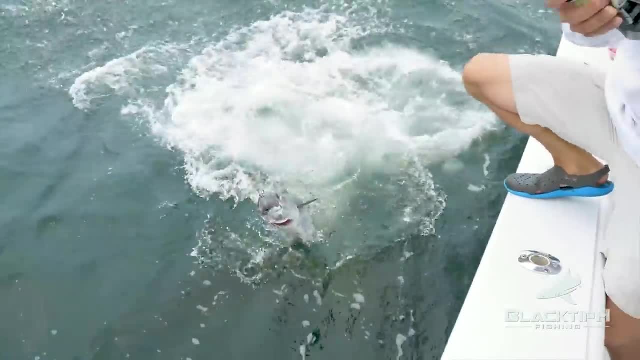 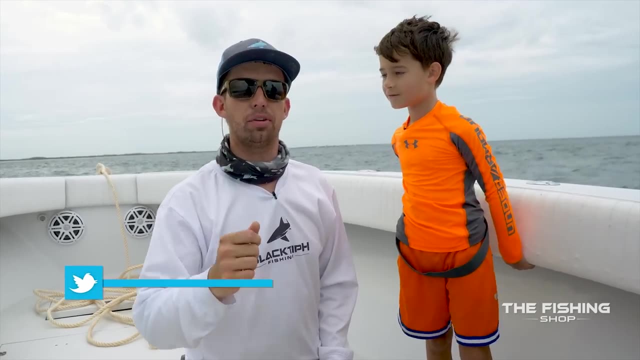 Here he comes. Oh, three of them at once. Oh my gosh, Oh jeez. Food chain challenge update. We got our first round of baits with just a plain hook, Vy. good job on that. We got the Bonita. Now it's time to catch a dinosaur. You saw those Goliath? 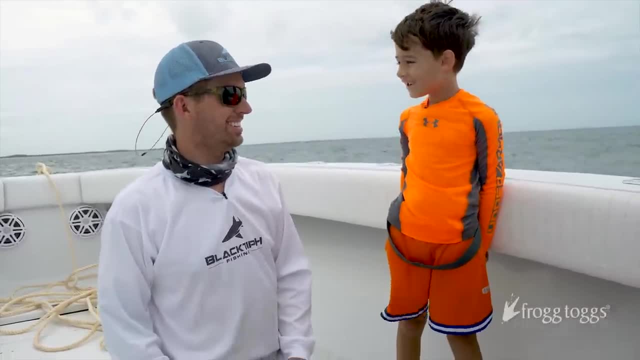 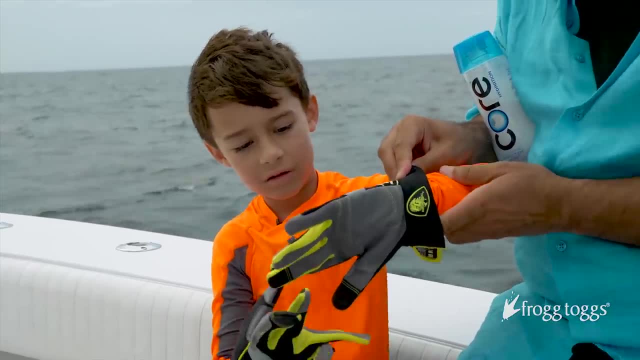 right, Let's go do it. Let's go do it. In order to catch a giant fish, you need a giant hook. What do you think, Vy? You think that's big enough. Yeah, You think we're going to get a Goliath with. 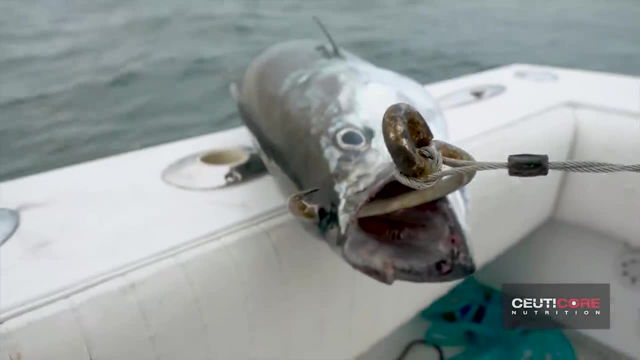 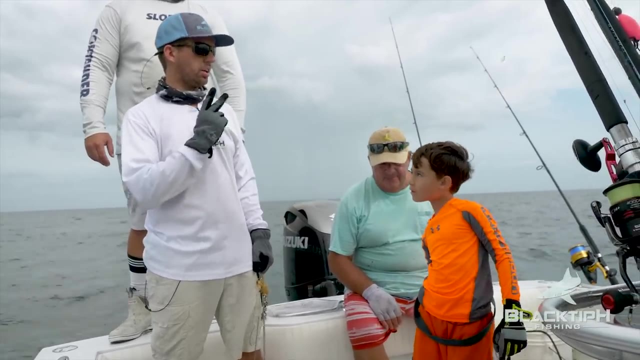 that? Yeah, All right, Here we go, Ready, Got a big bait too. So, Vy, there's two rules for hand lining. Number one: never step on the rope. Number two: don't get caught on the rope, Don't. 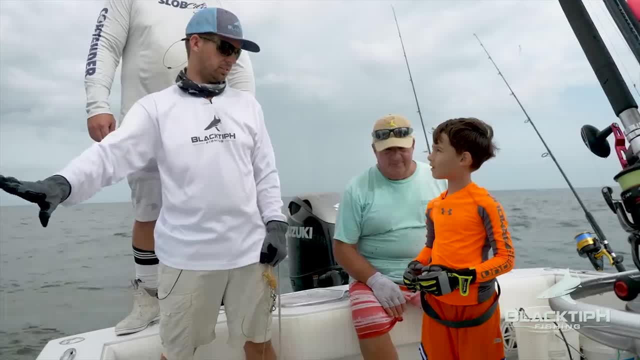 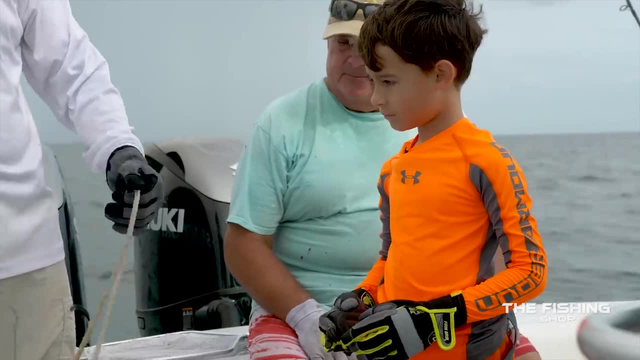 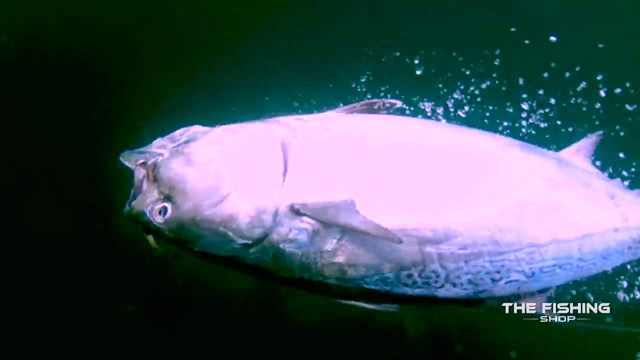 wrap your hand, Nothing. You want to let the rope just do its thing. So you're just going to hold on to the rope like this: You can just squeeze it with your fist. You don't want to wrap or anything like that, because you'll get pulled in You ready. All right, Here we go. I'm trying to make. 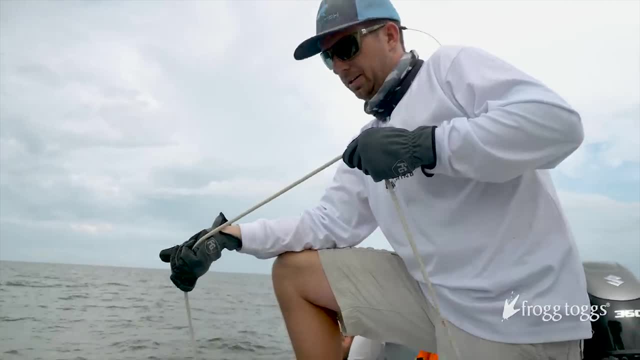 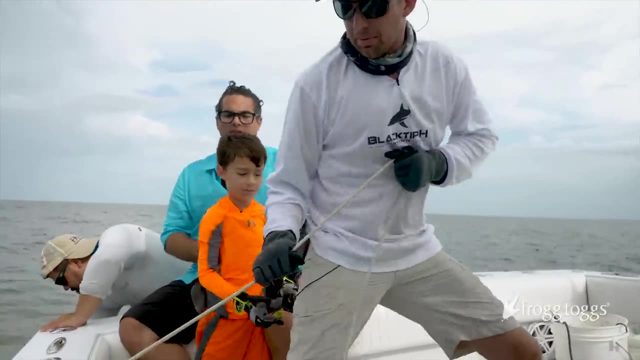 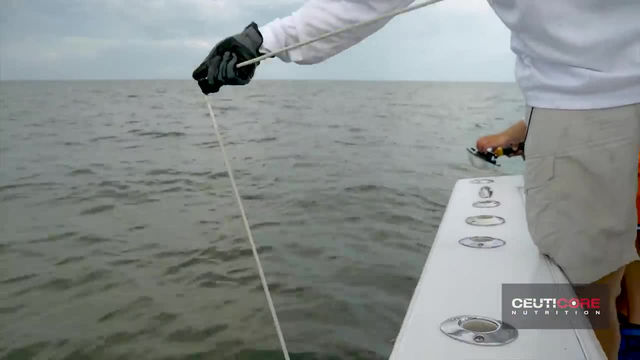 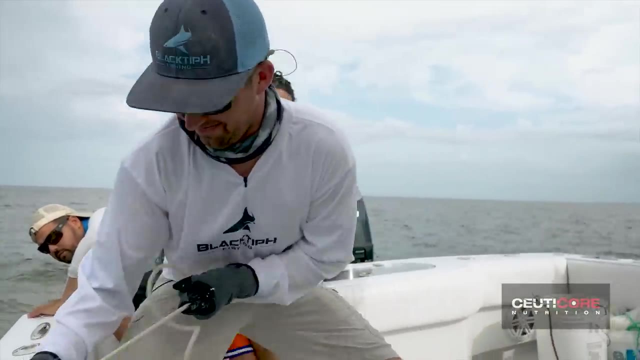 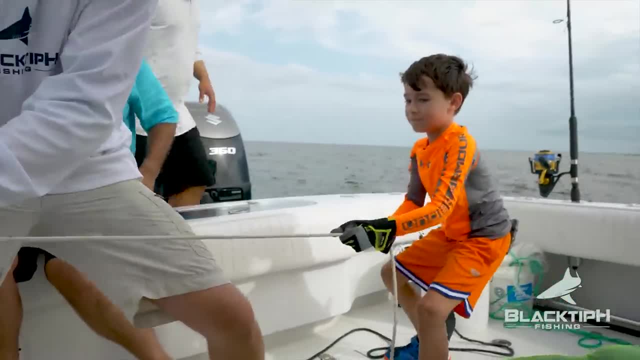 grab it Right there. Hold on tight, Hold on tight, Hold on tight. We got him, Come on Me and you, We got him, Come on Vy. Pull, Pull, Wait, He spit it, He spit it. I don't believe they can. 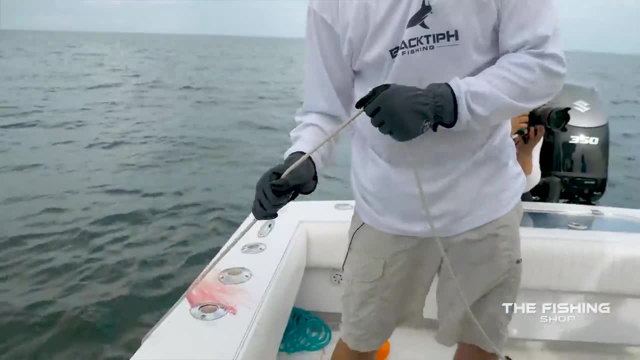 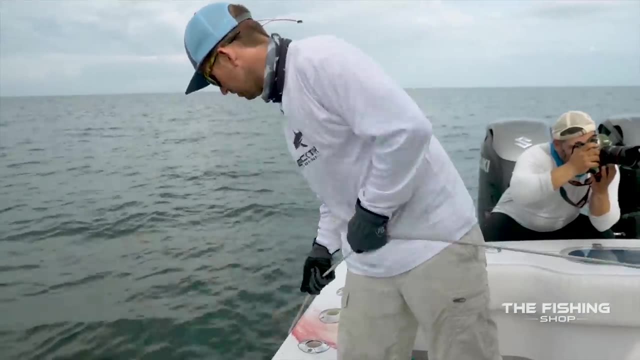 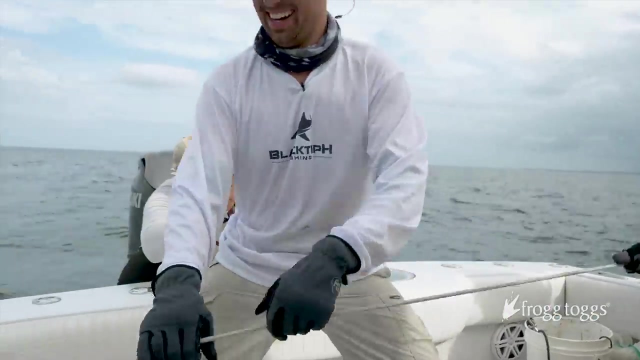 hold it that hard, Oh, he ate it again Ready And wait. No, no, He spit it. Oh, daddy, just got it. Oh, my gosh, Pull on, Pull, pull, Pull. We got him. Come on, Chris, you got it. 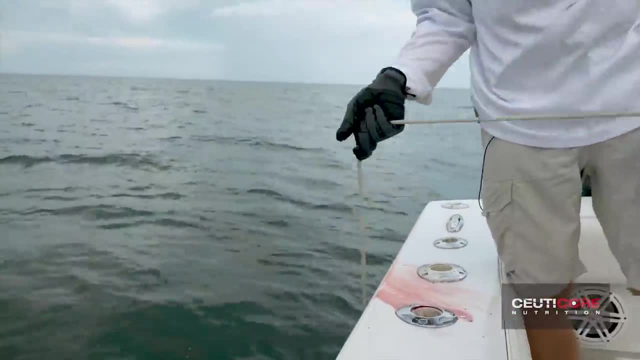 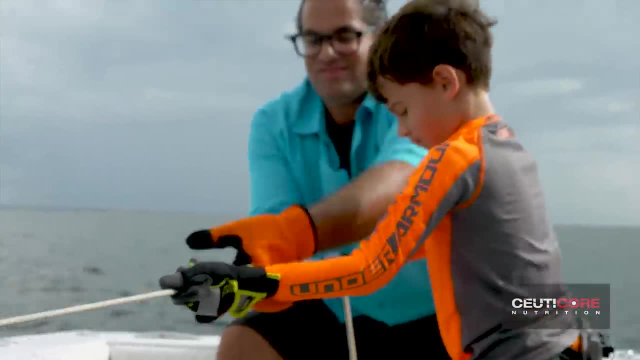 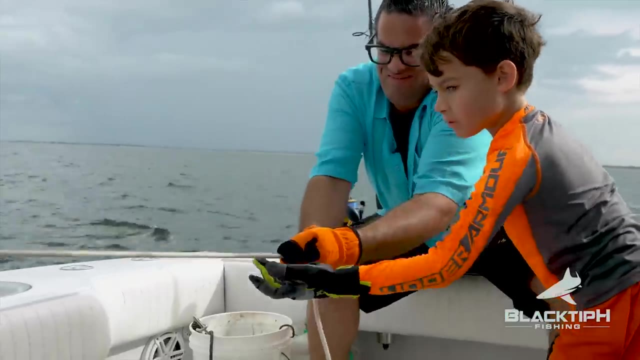 We got him. Come on, guys. come on, come on, They're not Pagani gloves. Come on, V. hold on, man. You gotta help us out. Come on, V Dude, that's a big one, bro. 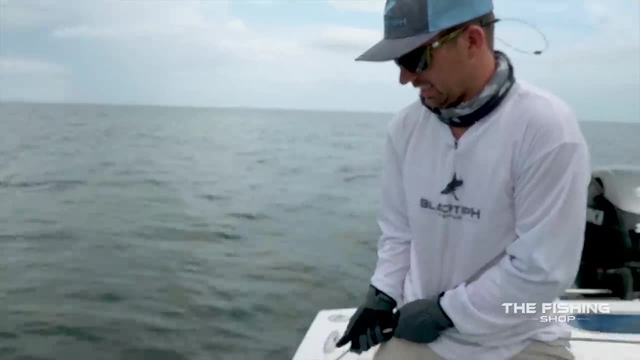 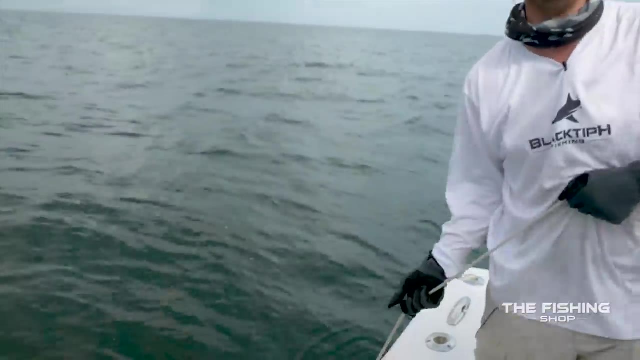 Is it? Yeah, it's over 400 pounds. Hold it. I hear that noise. Oh, he's so big. Oh, my gosh, Chris, he's giant V, he's a monster. No, no, no, no, no, no. 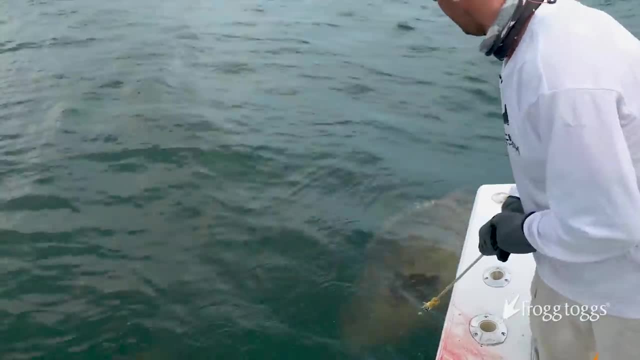 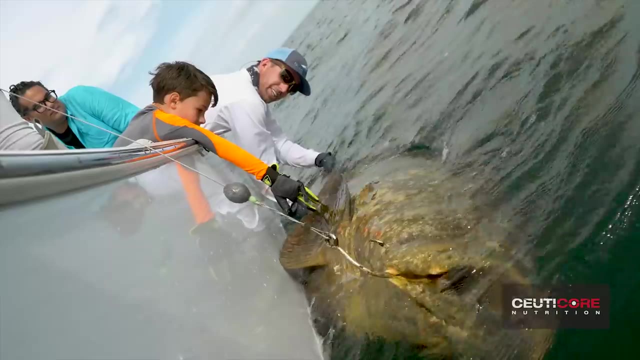 He's giant dude. Come here, Come here. V Come here, look Look at him. V Come here, Come here. Look what we just caught. The food chain challenge is complete, folks. There's nothing bigger than this in the ocean. 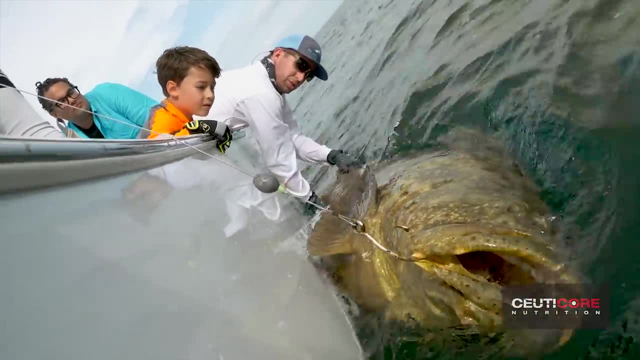 I can eat this thing. So we're from Bear Hook, Here we go. I'm gonna give this to a Threadfin, to a Bonita, to this monster right here. Gonna, let him go. Hey, he took my glove, man. 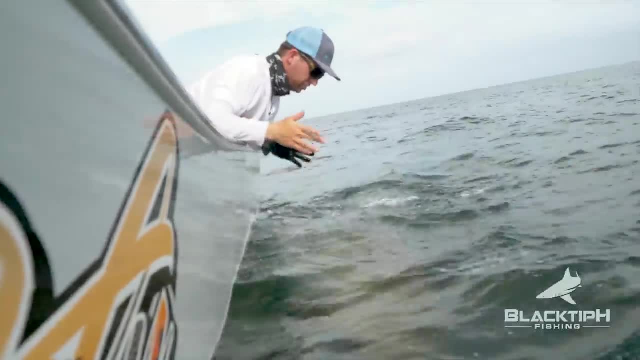 He's still eating it, Man, he ate my glove. Guys, he got a little bit of fiber there with these gloves. I mean, I don't know how much nutrients is in these things, but I'm missing a glove now. It's okay though. 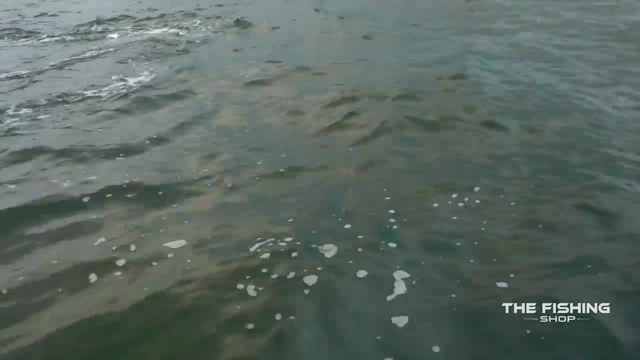 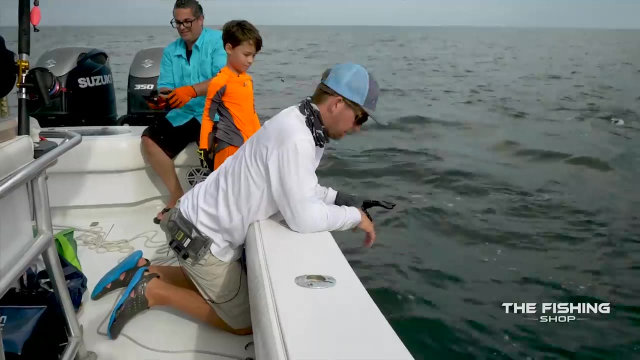 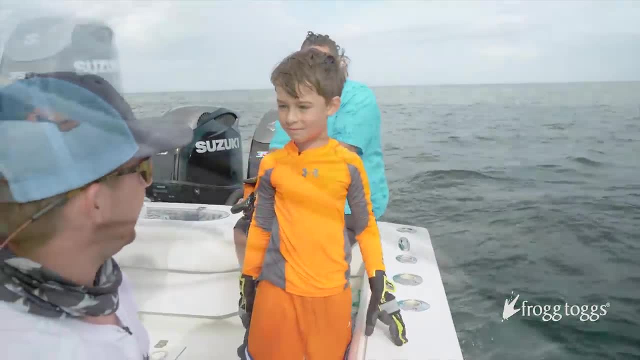 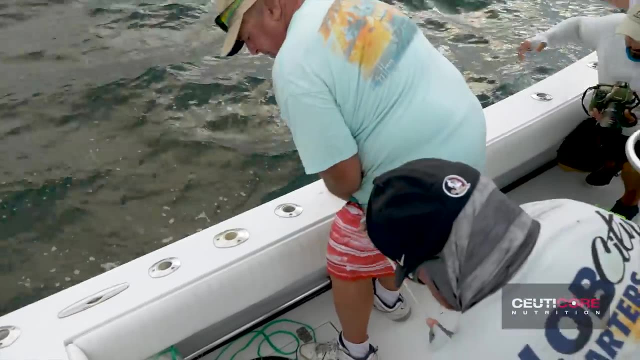 We did it. We did it. V, we did it. bro, Come on, Carl, Uh, oh, uh, oh, Uh oh. Come on, guys, Stop him, Stop him, Stop him. You need a spot, Hey. 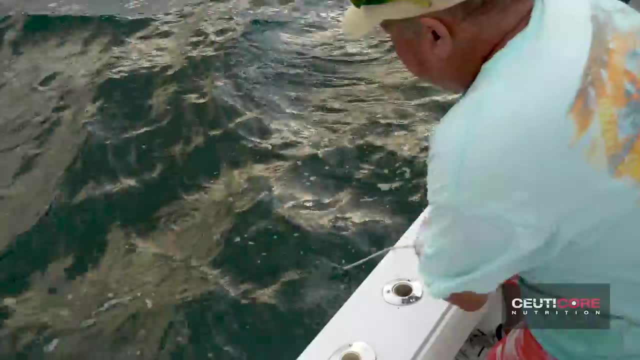 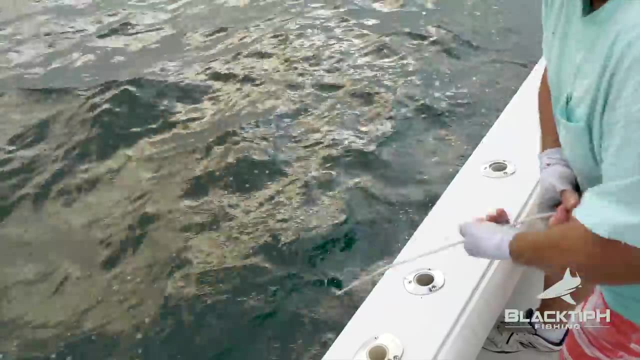 He gains the right compotion. How your hands, They feel fine. Yeah, They do. Come on, Carl, Stop him. Oh, Oh, my God, Here we go. Look at that, Look at that, Look at that. 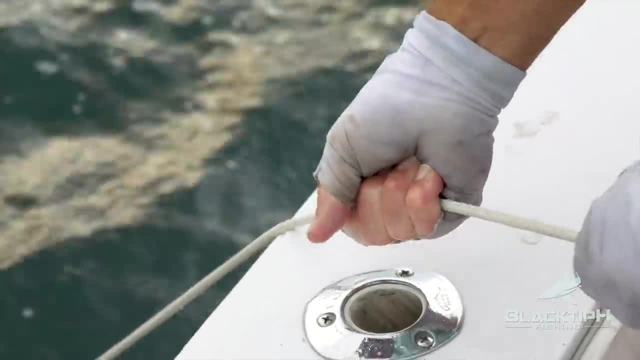 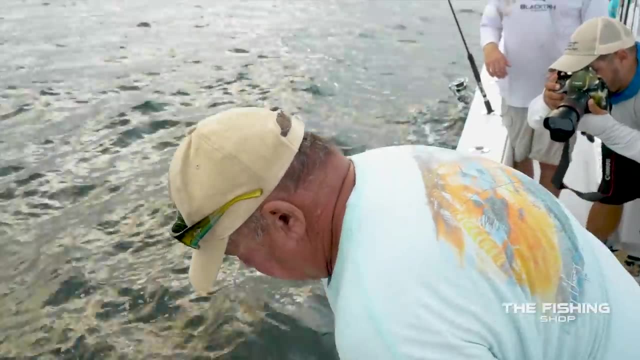 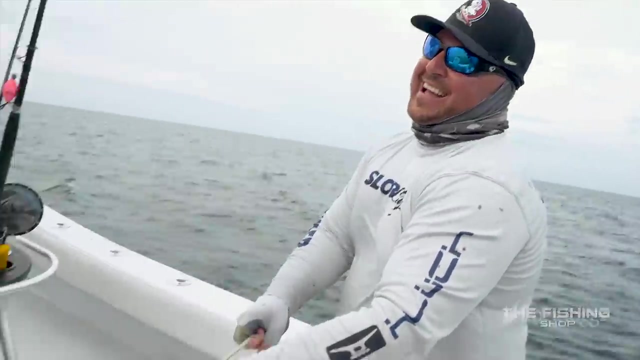 Waa, Look at that, Look at that, Look at that. Oh, my, My hands are burning. I don't have finger potato. How much has your hands hurt? I have finger potato. Your back's hurting. Yeah, I'm coming in, boys. 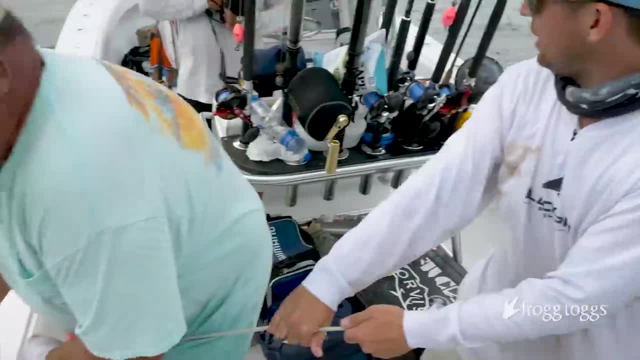 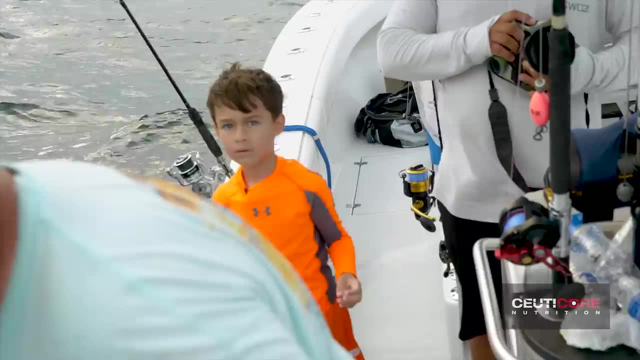 I'm coming in. Reinforcements are here. Let's go. V V, come help us. We got the big one on In the rack. He might be. Aw, you guys lost my $70 rig. I don't know if you're trying. 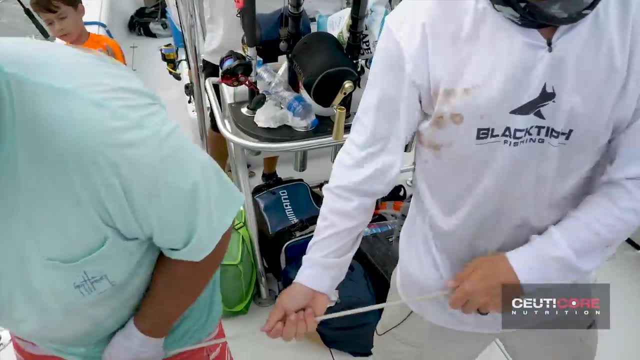 No, don't let go. Don't let go. He's still there. Pull him up. He's still there. He's still there, He's still pulling. Pull, pull, pull. We need to pull. Come on, let's go. 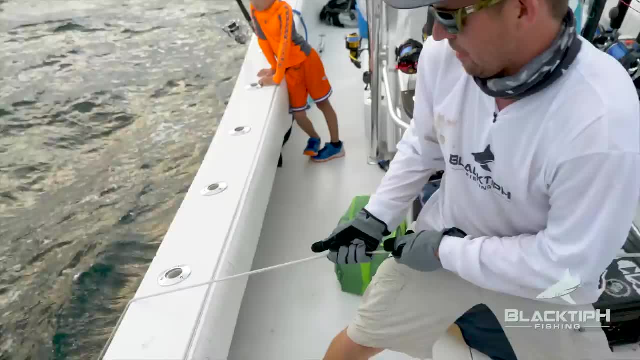 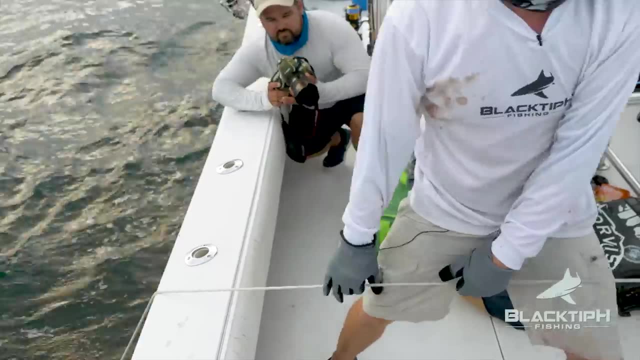 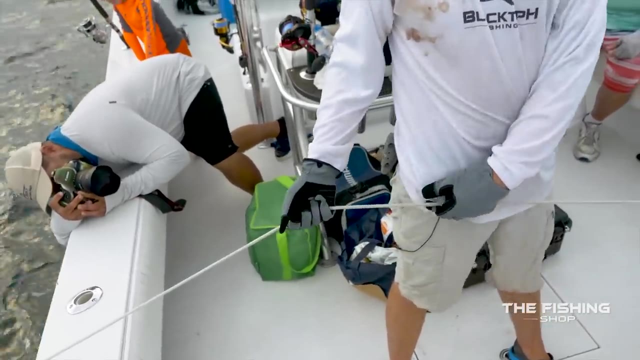 He's going to come out, bro, Come on, Come on, I'm sure he's a strong guy, Bro, he's pulling the whole boat. Yeah, you're just in the rack, Bro. this is an actual invoice. This is nice. 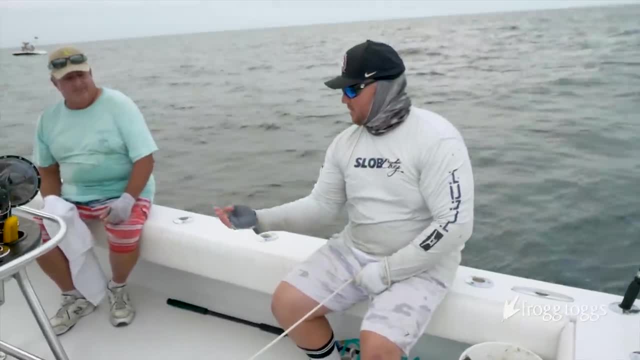 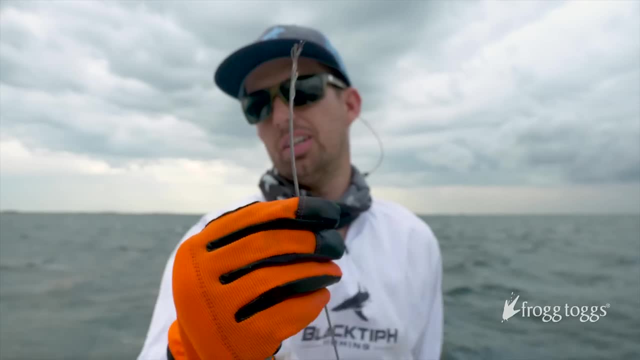 It's called Earth. It doesn't move. We got whitecaps on the horizon. We got to head in for safety, But we had a great day in the water here, guys. Thanks so much, Steve. Yeah, thank you Got some big fish. 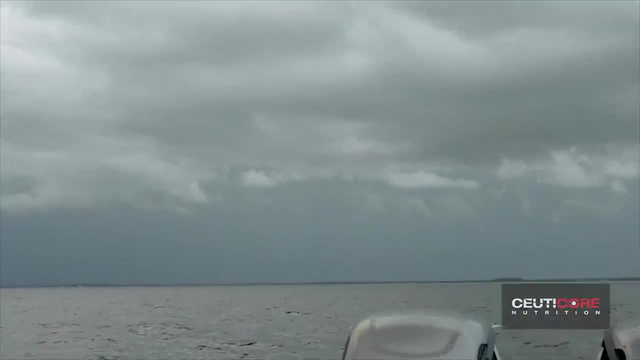 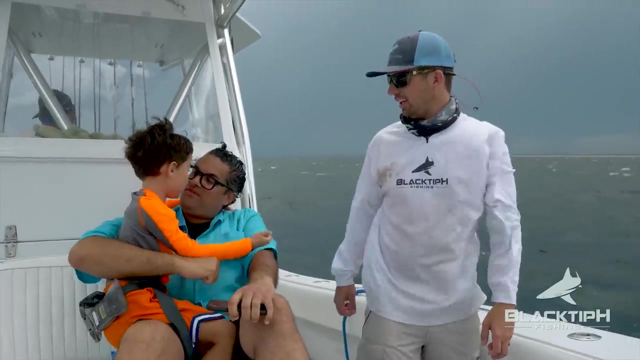